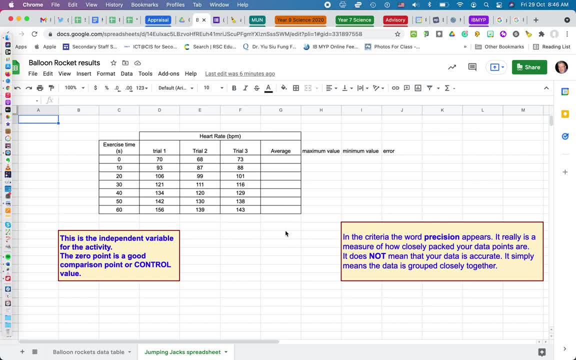 Let's say I've got there and have a data table that looks something like this: I've done my exercise time and I have my heart rate and notice everything's labeled and notice I've only got numbers down here. Now please also notice I've put some little reminders here. This column will 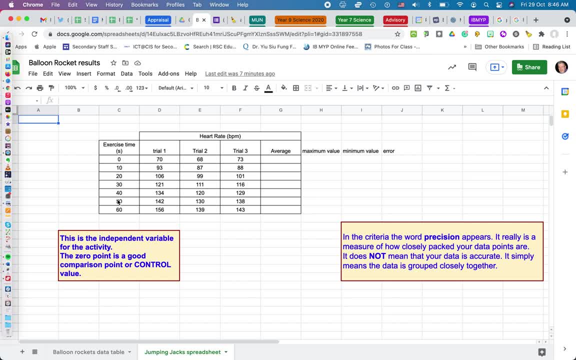 be my independent variable. This is the best way to set it up. Here is my dependent variable. I have trials and I have enough data to make sure that it's reliable. Now one of the first things we need to do is to think about how to do an average. I should have set this up before we started That. 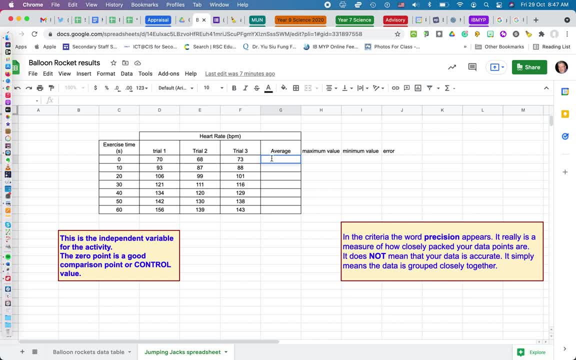 was very remiss of me, but I didn't. So what I'm going to do is very quickly do it now To tell the machine I wanted to do something. I type in equals Now because I've been working with averages quite a bit. it has come up with that. But if I had not been working with averages, I would type in AVER and I. 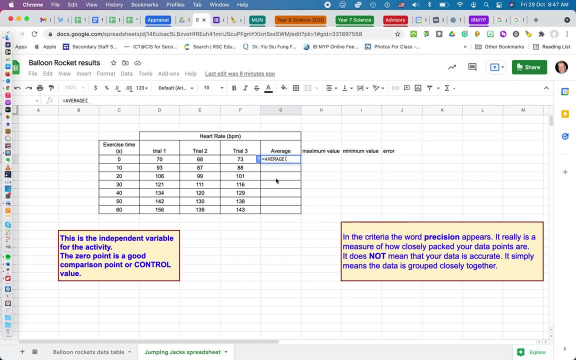 would get this come out. Then if I go to average, then I can simply tell it what I want to average. I'm going to say I want to average these three numbers, Then close the bracket Right. once I've done that, it will do the same thing. I'm going to close the bracket. I'm going to close the bracket. 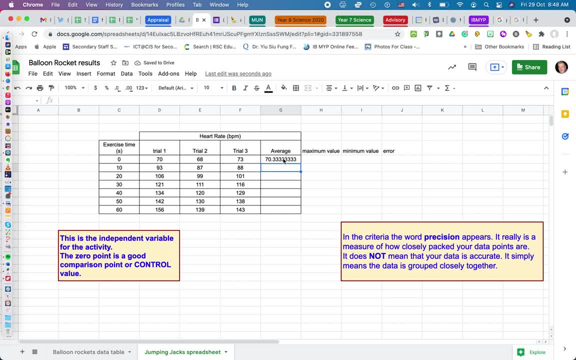 Once I've done that, it will do the same thing. Once I've done that, it will do the same thing. That's my average. Now, if I want to do the same thing below, I don't have to redo that sum. All I have to do is: 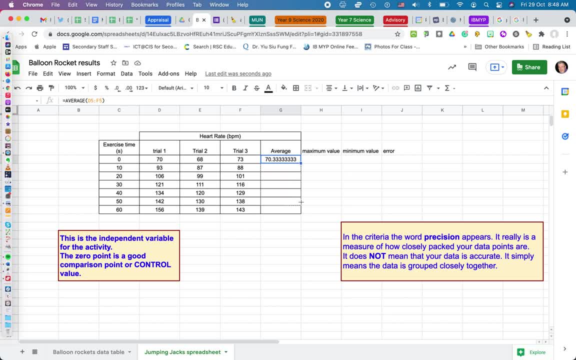 to grab this corner and drag down. I have now done exactly the same thing. Now, what I would suggest you is that you always keep the number of decimal places in your average the same as it is in your trial data. So we come up to the top and decrease. 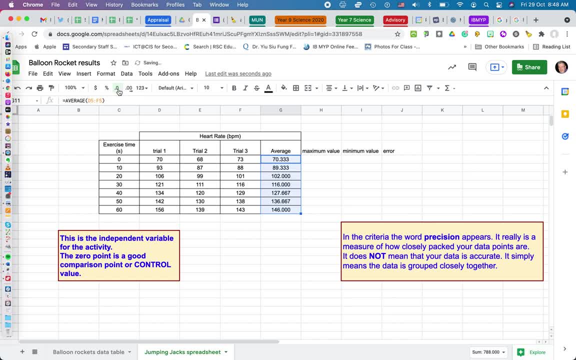 and, as you can see, I'm gradually rounding and decreasing, or rather the machine is rounding for me and it makes sense that heart rate is in whole numbers. Right, that is where I've got to to start off with, but I'm not going to ask you, or I'd like you to also add a few other things. so let's get the. 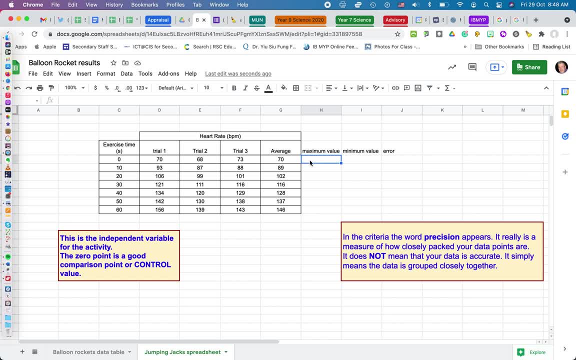 computer do it for us. Now I want to know the maximum value in each of my rows. so again, I'll type in equals. If I type in max, it asks me: do I want the maximum figure? and I sure do. Highlight the trials. close the bracket and hit enter. 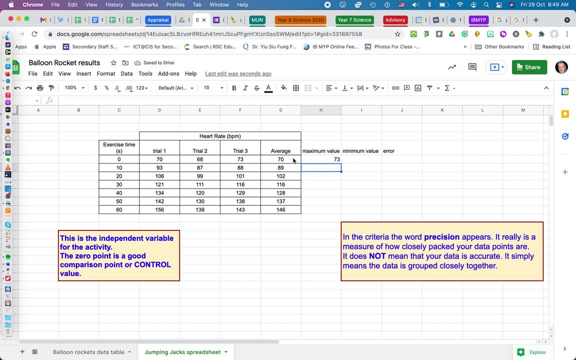 So it will get the maximum value for me. Now, if I copy down, it's done it for all. Let's do the same with minimum instead of typing max. type min, Tell it what you want to do, Hit, enter, copy down. Now this year we're going to look at the thing. 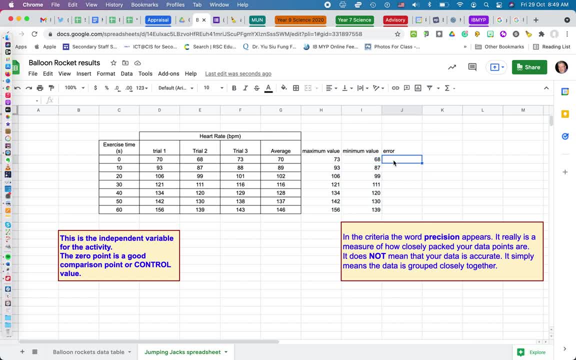 called error, and error is a simple calculation we're going to use and it's the maximum value minus the minimum value and divided by 2.. So let's put that in, so it's equals this number. click on it, hold on before I start a bit, put some brackets. remember your math, That number. 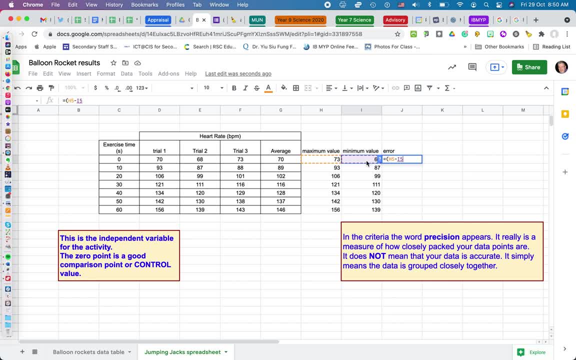 maximum minus the minimum. close the brackets forward. slash means divide 2.. All right, there we go. now you'll notice down the bottom I'll put in a little box here which talks about precision, and this is something you need to comment on in your